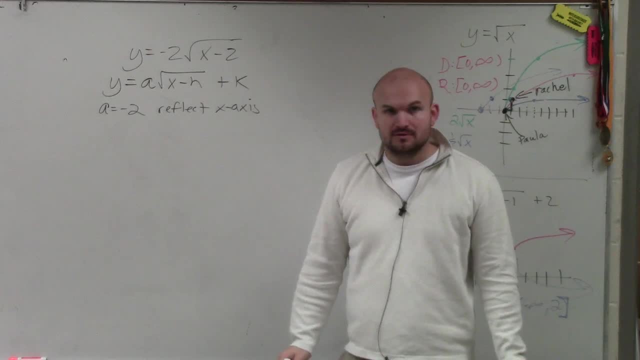 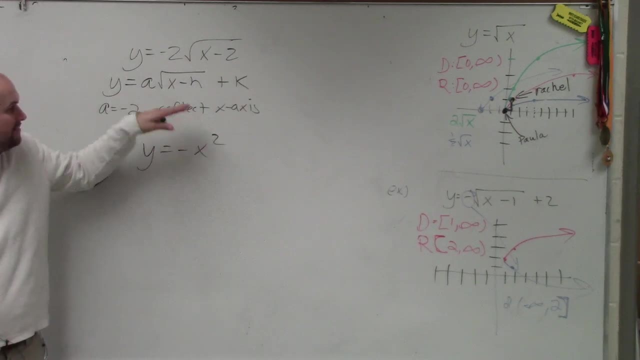 that's a reflection of the x-axis, right? You guys remember that Right? Anytime you take your function and multiply it by a negative, that's reflecting about the x-axis. Okay, Then we have the x minus two. So your h is equal to two, Because it's x minus h, X. 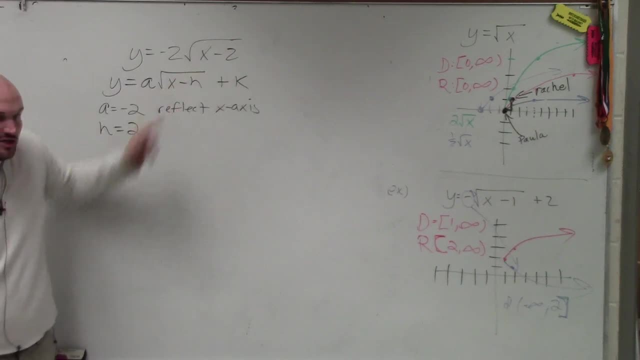 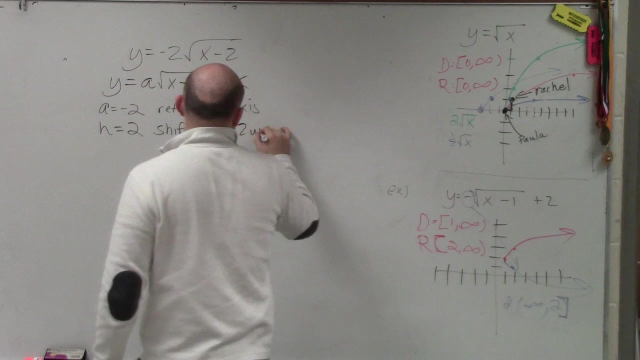 minus two, So you're minusing h. H is two. So since h is equal to two, you're going to shift right two units And I'm sorry, this is a reflect to the x-axis as well as. 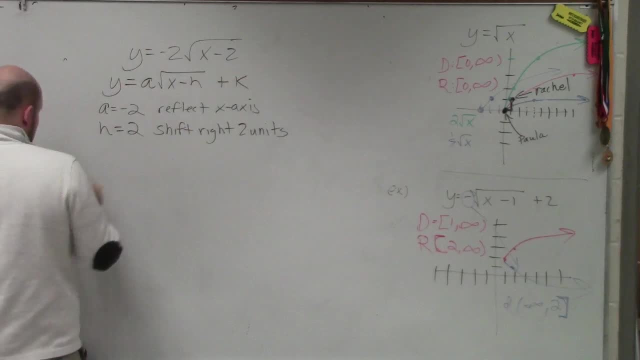 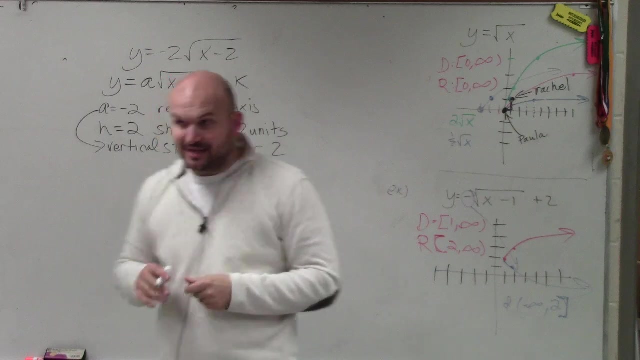 two is going to be a vertical compression- I should have written that in there, I'm sorry- a vertical stretch, So a, if it's negative, reflects it. about the x-axis, It also talks about its vertical stretch, which, again, I will explain here in just a second. So to graph this the most: 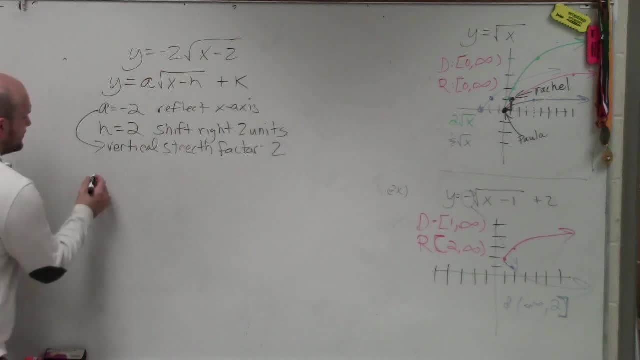 important thing in my opinion, is to know what the parent graph looks like, And the reason why I showed you guys this is when you're in the parent graph, you guys can create a table, or you can kind of take my word for it. We understand that you cannot use negative. 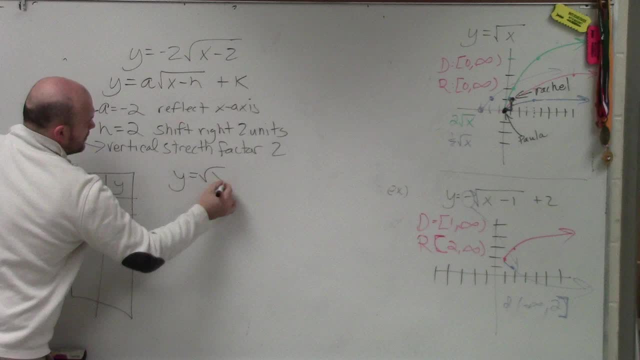 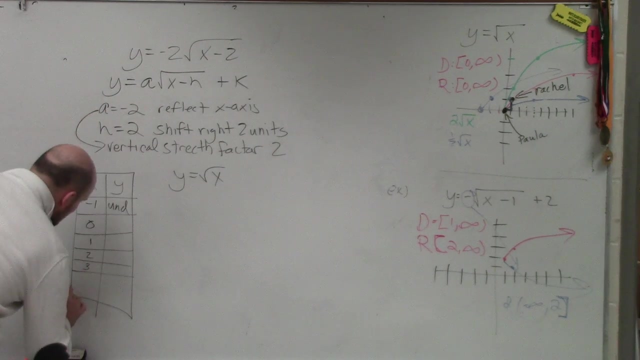 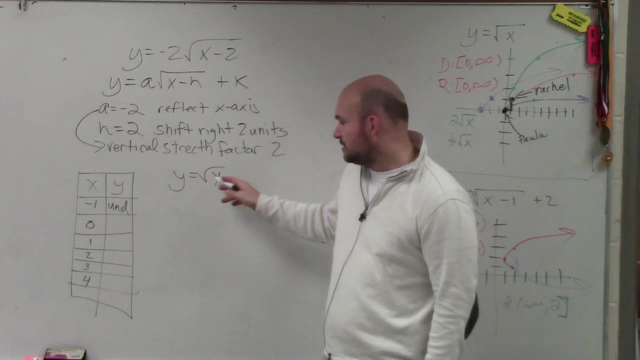 numbers into this function. Right, You can't plug in a negative number. That is undefined, Correct. Okay, So we start picking numbers. Zero One. Now I would not choose the numbers two and three, Because, can you take, when you plug in one, let's plug them in Zero. Square root of zero is: 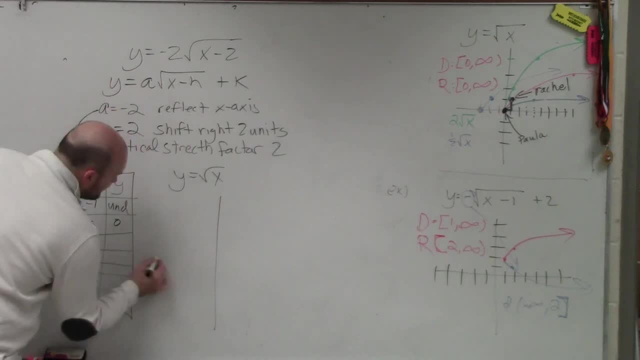 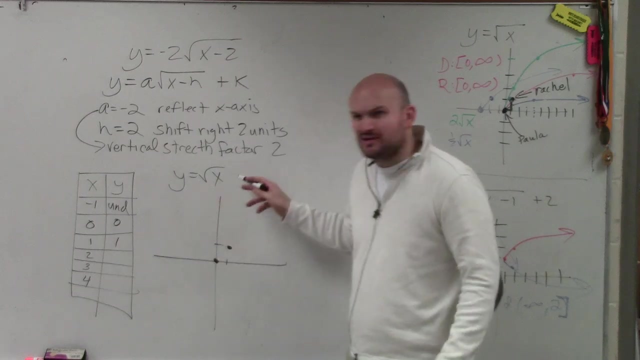 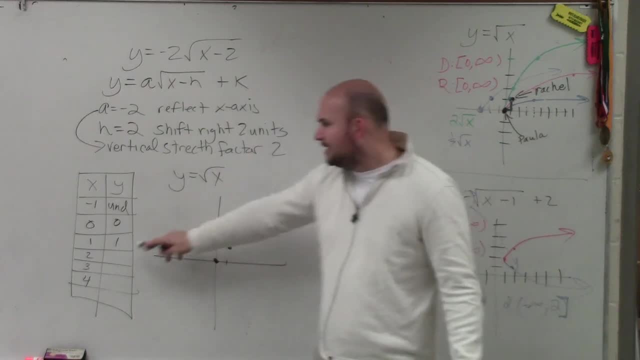 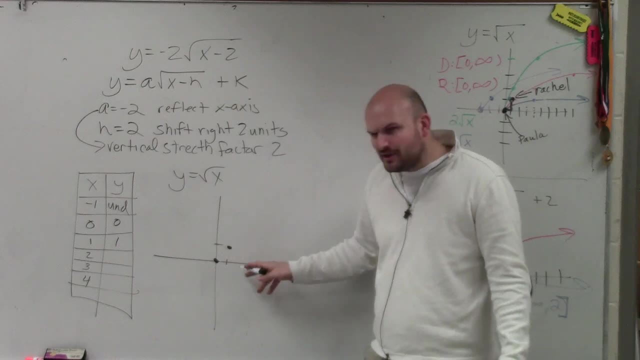 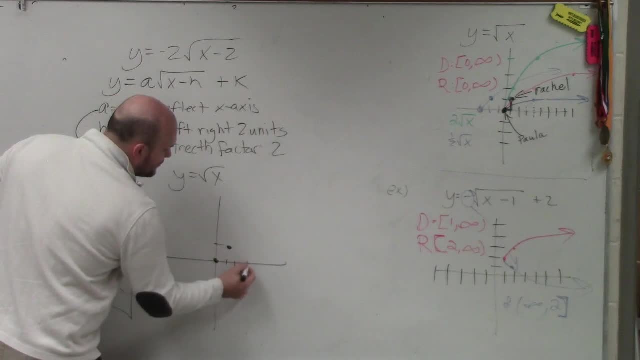 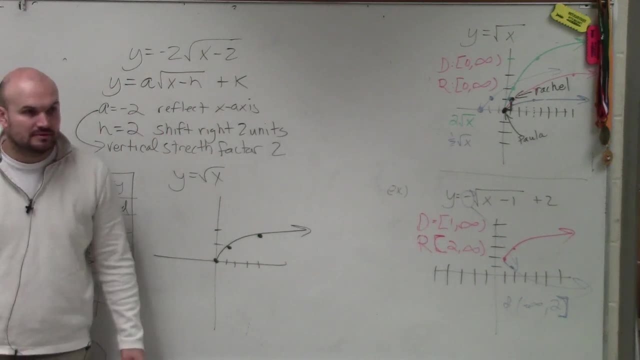 what's the square root of 4? 2.. 1,, 2,, 3,, 4.. Does having these points kind of give me a good idea of what the graph looks like? That's with no transformations. That's what we call. 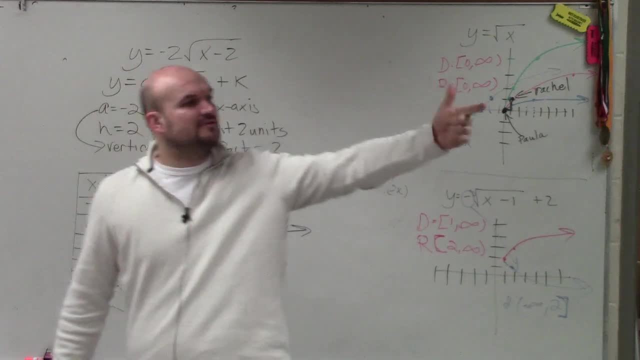 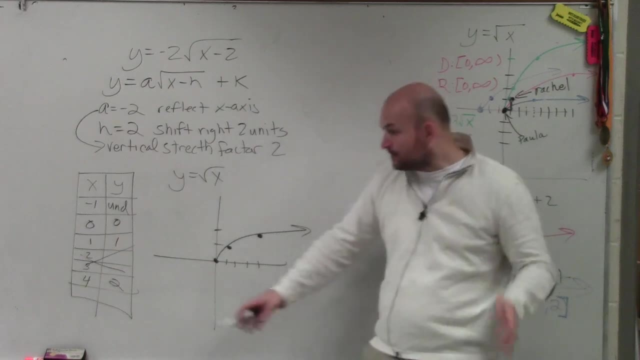 the parent graph And you guys should be able to do that. for a quadratic, an absolute value and a cubic function, All you have to do is create a table. But sometimes you want to create a table, you want to choose values And, if you guys remember, I didn't plug in 2 and 3. 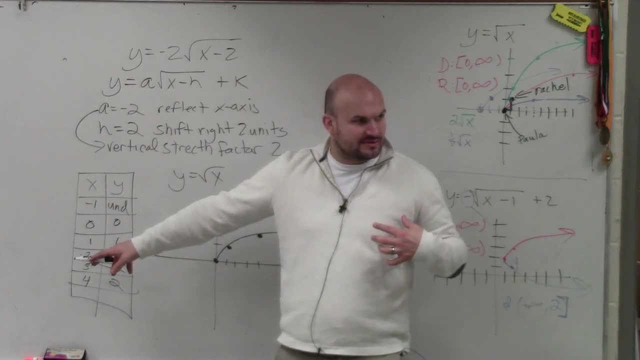 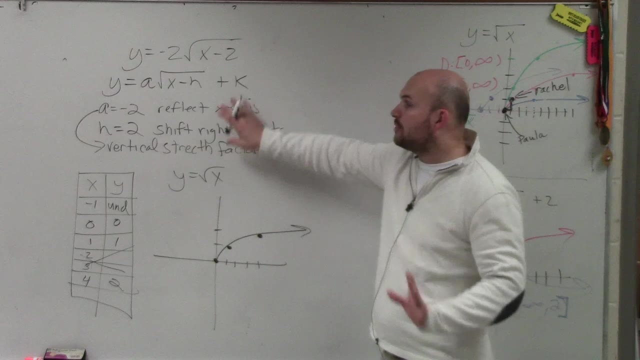 when I chose my values right. I chose the values, I chose 0,, 1,, 4, and I chose 9 as well, because those are points that make sense. So now all we're going to do is go back to our factors. 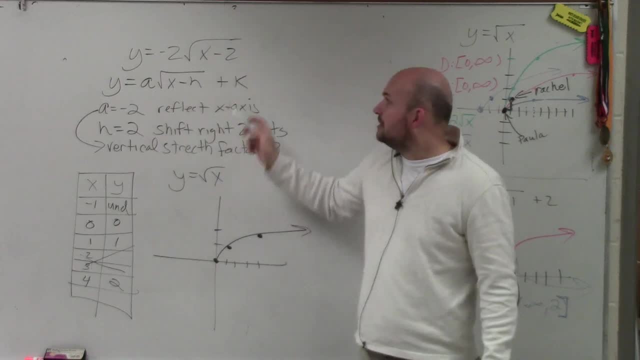 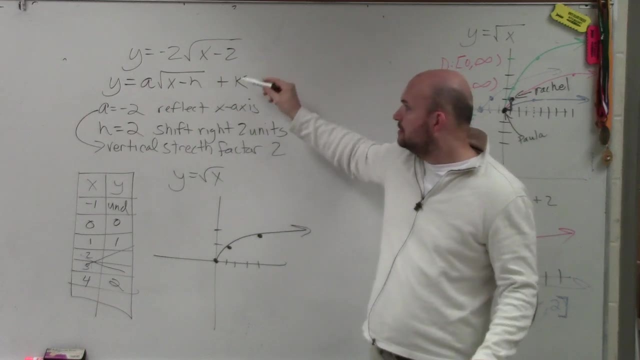 So what's happening to this graph? Or let's go back to our transformations. Is this graph being shifted at all, left or right? Yeah, it's being shifted where: Two units to the right, Two units to the right, So all in total. 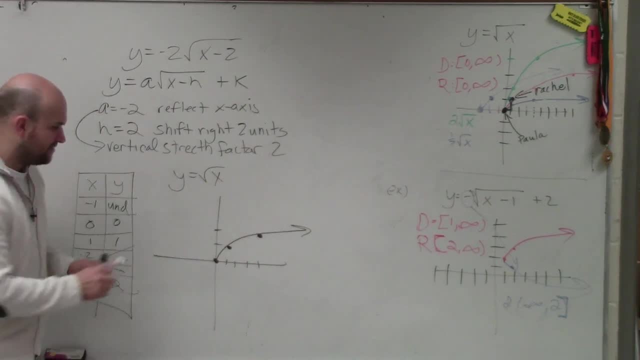 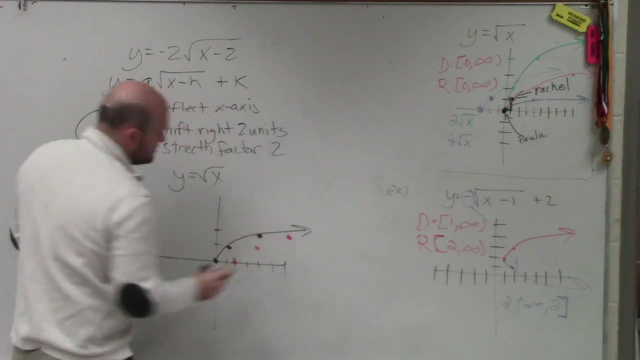 So what I'm simply going to do is take each of my two points that I found, and I'm just going to move them two points to the right. Does that make sense? Yes, Does that make sense? Okay, Then what else is happening to the graph? 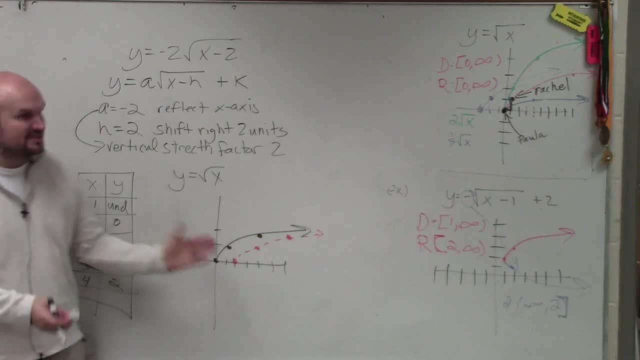 Well, the graph is now being reflected about the x-axis. So, instead of the graph going up, it's now being reflected down. So now, all of the points that I just found I'm going to reflect about the x-axis. So, instead of the graph going up, it's now being reflected down. So now, all of the points that I just found I'm going to reflect about the x-axis. 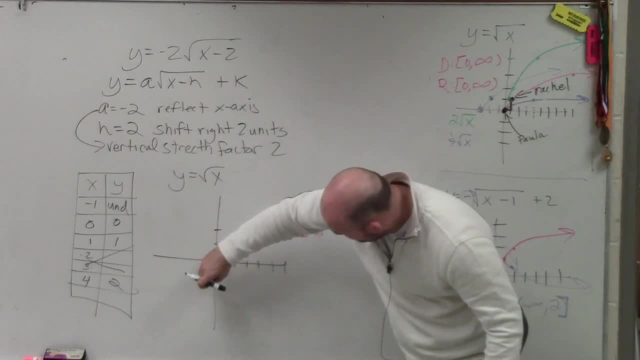 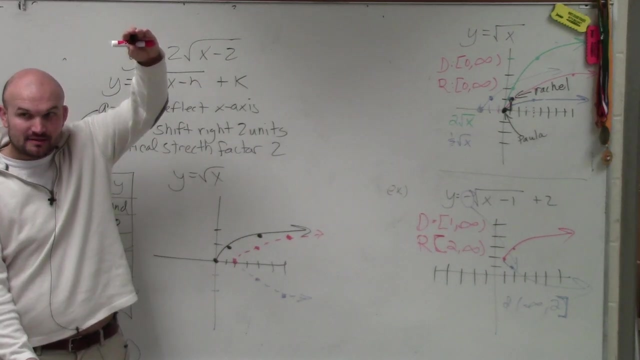 the x-axis. So instead of going up, I'm now going to go down. Does everybody see how my graph is now being reflected? Yes, And then the last thing is is being there's a factor of two. You're vertically stretching the graph right. Vertically stretching- Yes, Do you guys remember? 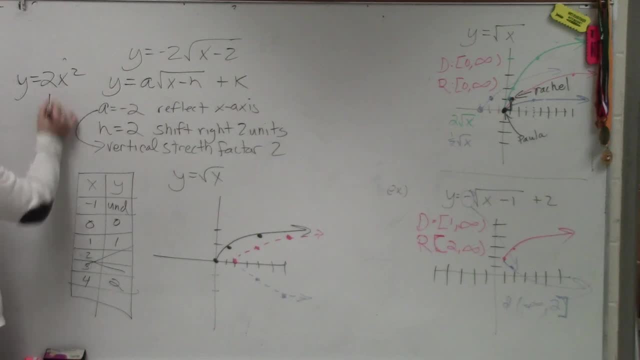 y equals two x squared. What did that do? That made the graph look skinny. right, It vertically stretched the graph. So how does that do that? Well, basically, all that two does is multiply all of your y values by two. You're basically just multiplying each of these y values by two.